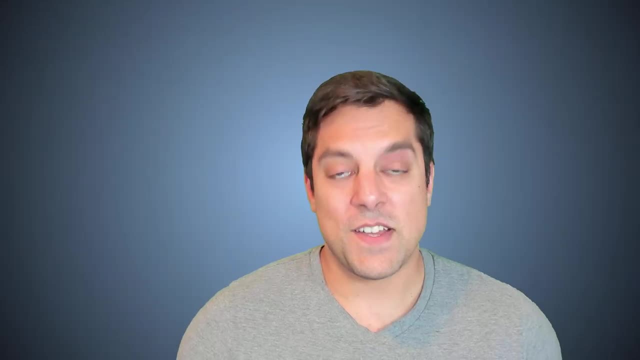 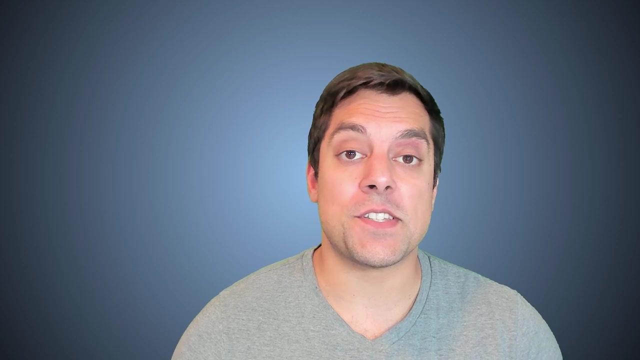 What's going on, folks? it's Mike here, and today I'm going to be talking about another design pattern, This time a behavioral pattern, which is known as the iterator pattern. Now, this one itself almost speaks to itself, So let's go ahead and just dive in and we'll. 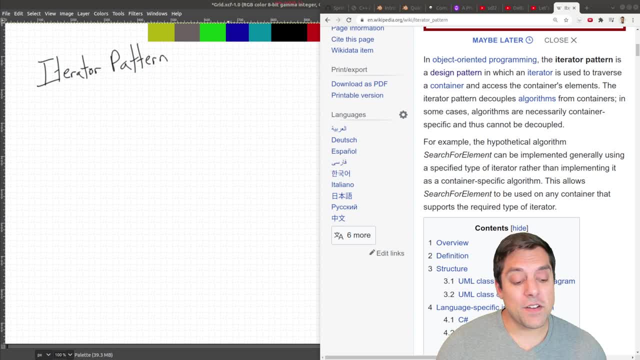 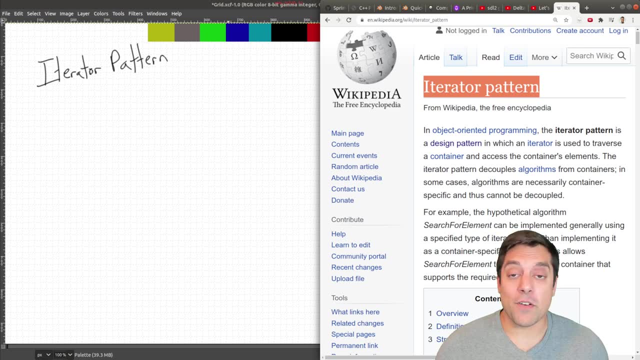 take a look at the iterator pattern to learn more. So the iterator pattern itself here is quite useful in the sense that you can use it, or are probably already using it- in your code. I think the Wikipedia article gives a nice introduction to what the pattern. 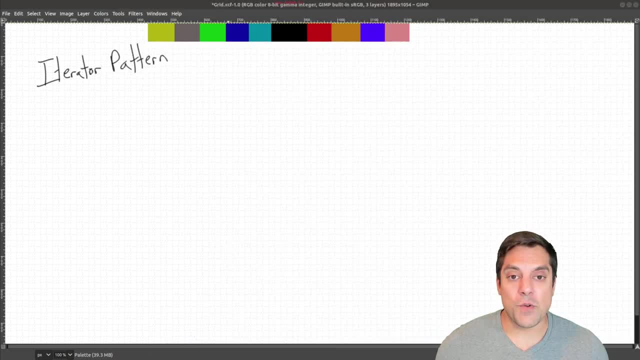 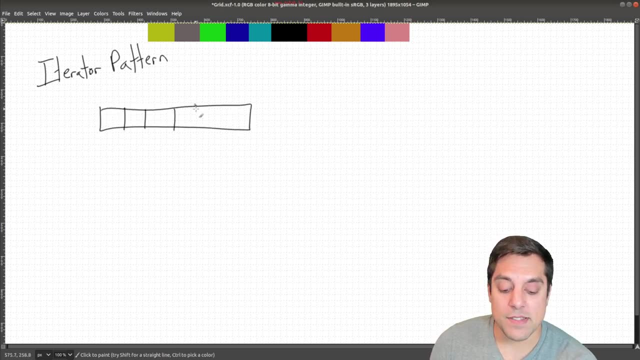 is, but I'd rather go ahead and just show you what the pattern is intuitively here. So the idea is, if you have some collection- maybe it's an array, maybe it's in a vector, maybe it's a tree data structure or something you know- less trivial here and the idea is you 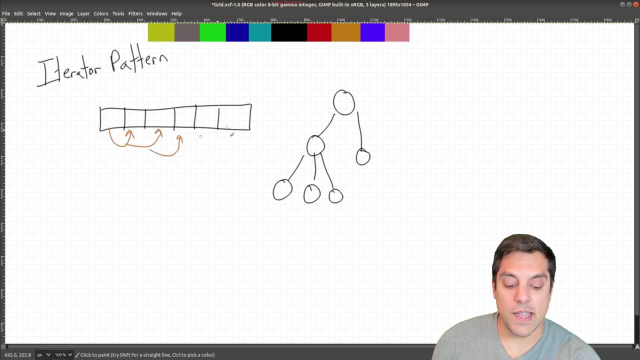 want to know how do you get to the next item and traverse this structure. So for an array, for instance, this might be pretty trivial to just move to the next item. but for a tree, we have many different types of tree traversals. Whether we're doing a 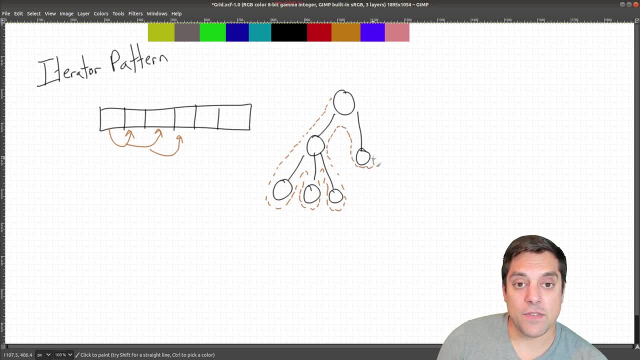 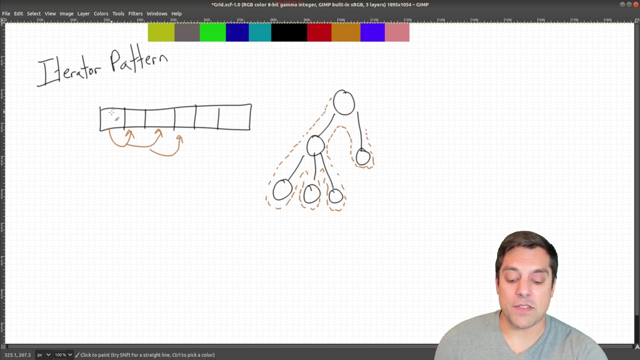 level order, a traversal, a sort of depth first traversal like I'm highlighting here, or a breadth first traversal. What you really want to know is that you have some consistent or uniform way to traverse a container structure. So again, whether that's a container structure. 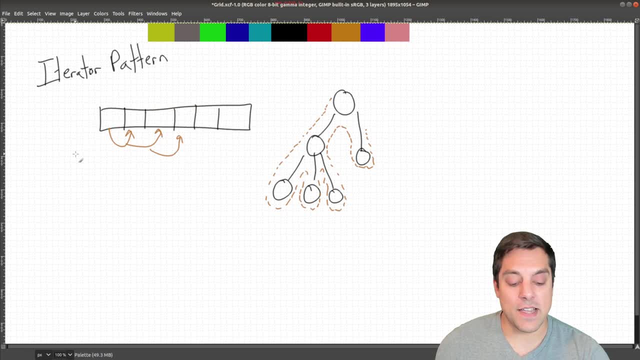 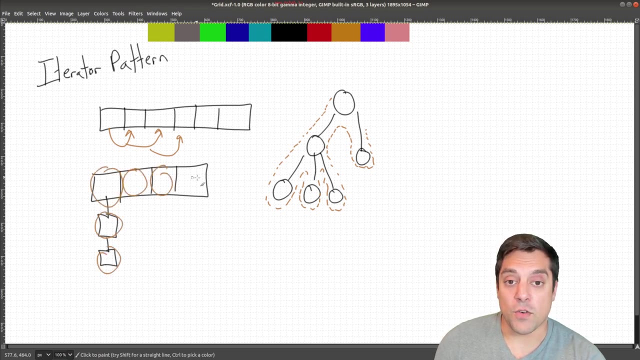 structure like this, using an array as a container, maybe a link structure like a tree or maybe some combination here, like if you have a change hash map data structure here, where you have to look through or traverse each of these buckets in some particular order. it's nice that that order is. 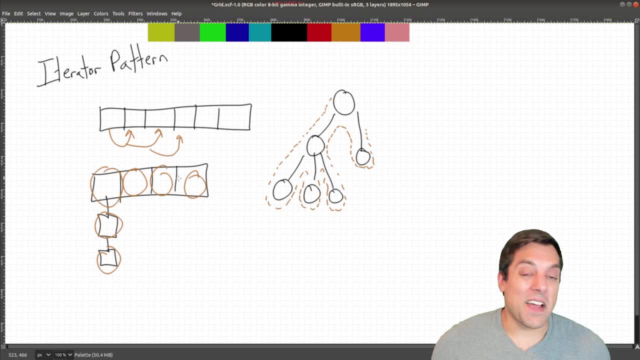 defined. so let's go ahead and just look at some examples here. i think you'll have some intuition, but it'll be useful just to see this pattern. perhaps in a future lesson i'll show how to design an iterator so you can get more of a feel of the design pattern. but for today i just want to. 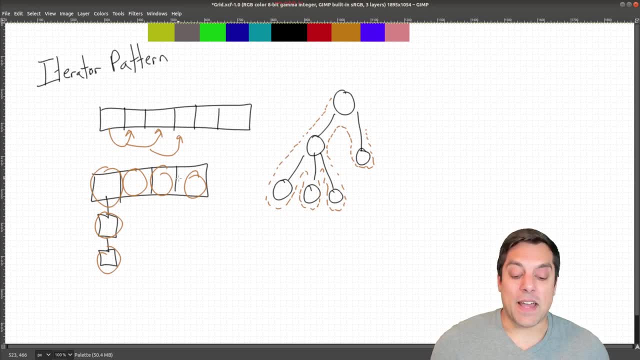 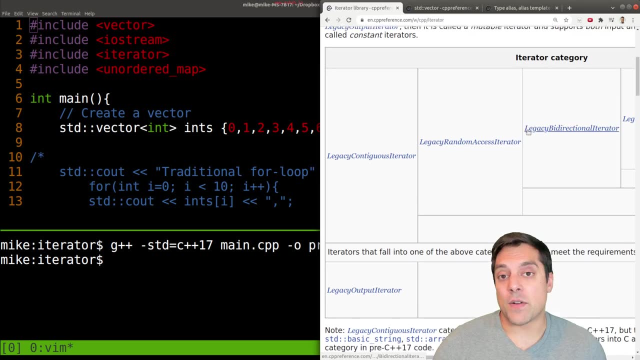 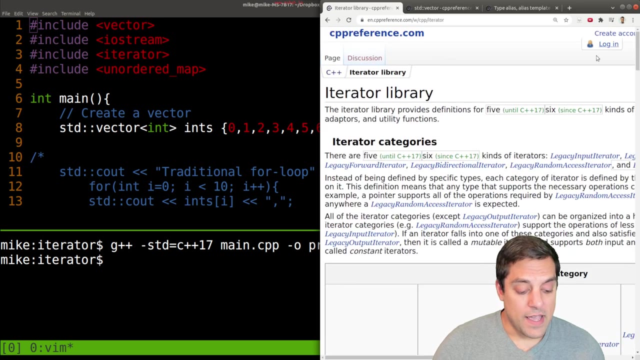 show you what's built into c++. so we understand the iterator pattern. now let's go ahead and look at what iterators are in the library, and we have many different ways to iterate: forward, backwards, bi-directional. in fact. there's six different iterators provided in c++, as of c++ 20, i believe. 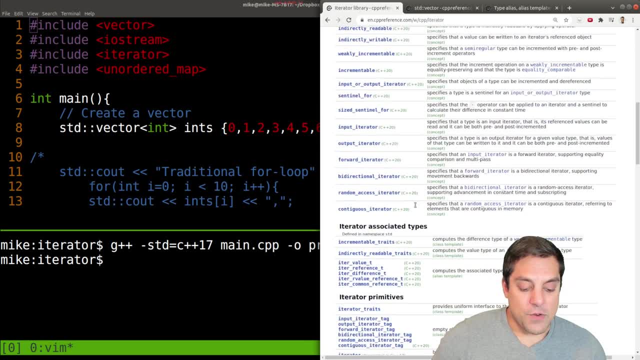 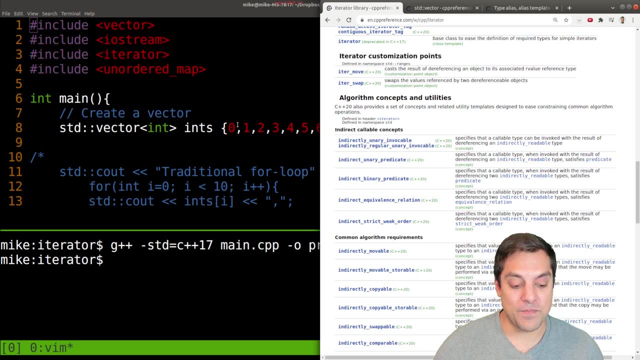 here or since c++ 17. so, with that said, we have quite a way that we can traverse data structures, but for this lesson, let's go ahead and just see how we can use them. so i'm going to go ahead and just start off with creating a vector. 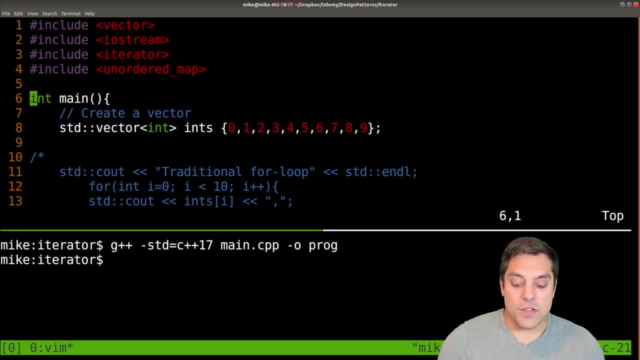 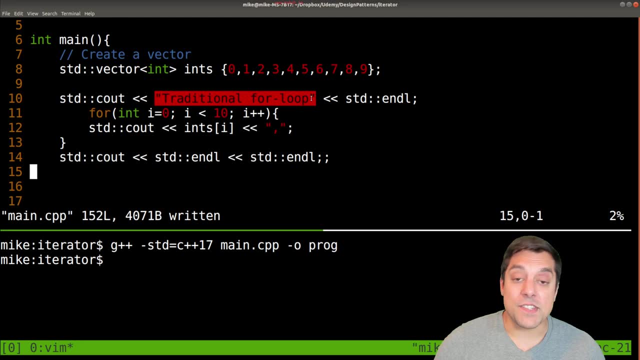 here of 10 integers and what i want to do is just take one code sample at a time and just show you how we iterate through data. and in this example, i have just a traditional for loop here and this is probably how you're traversing your data sets here. you have some loop here and you just specify hey. 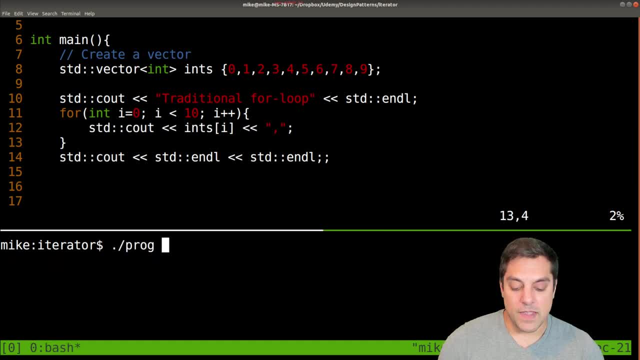 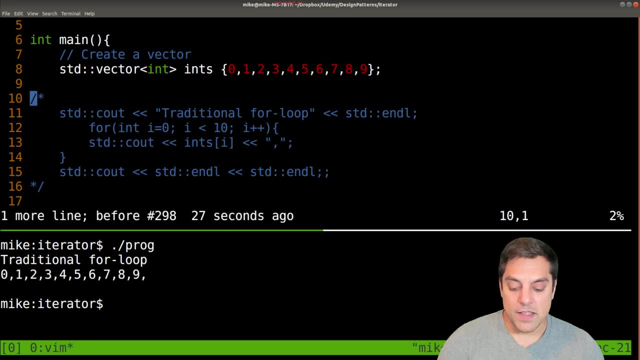 and i want to print them out. so let's go ahead and just run this and, as expected, you get your 10 elements here. so that's pretty obvious. so i'm going to go ahead and comment that out, and let's go ahead and look at another way that we can traverse this data structure or iterate through it. 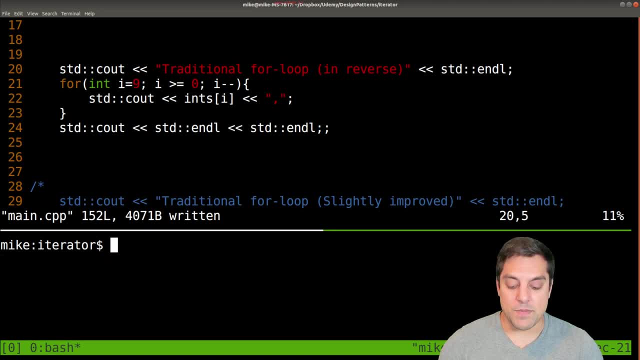 so we could also have a loop, just as we did before, but this time what's different is i'm traversing it backwards or in reverse. so if i go ahead and run this code, we'll see that we are traversing this data structure starting from the last element or the ninth element in our data. 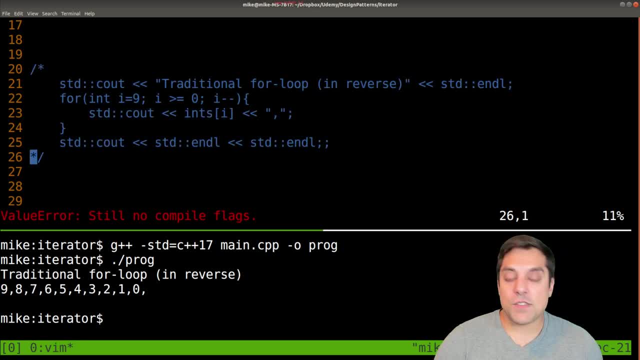 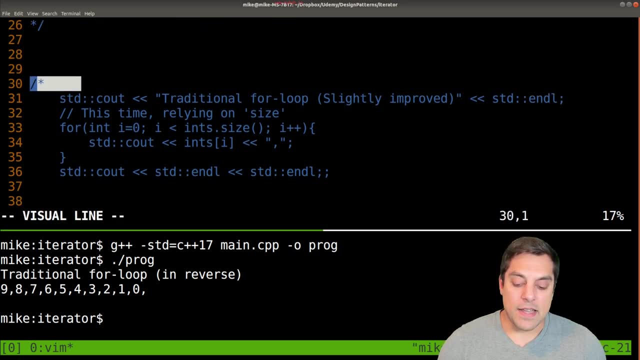 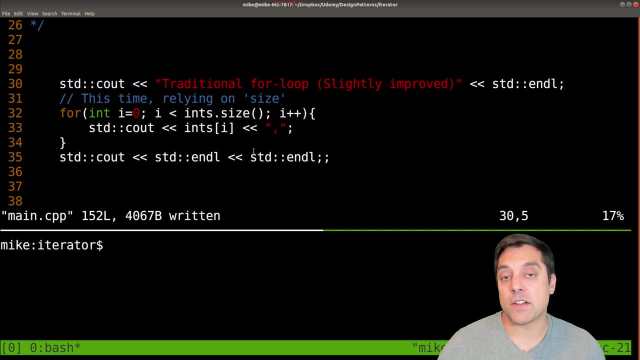 structure okay. so that's all well and good, but we probably want to improve this just a little bit more. so let's go ahead and create this iteration through our loop, but using something that specifies the actual container size. so in this case, for our vector, we have a dot size function that will allow. 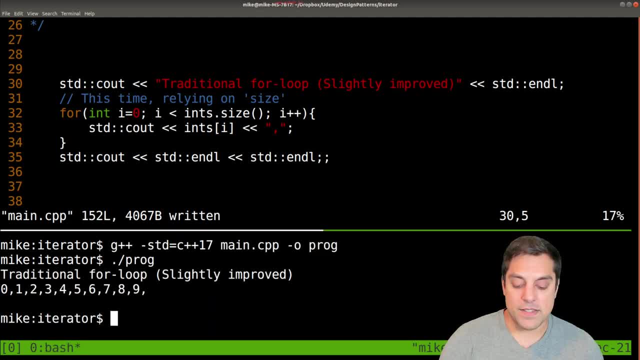 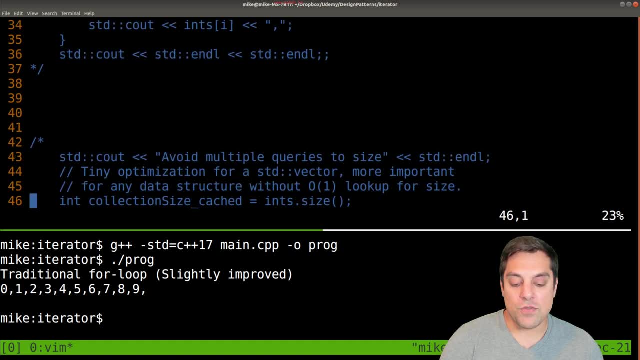 us to traverse our data structure. so i'll go ahead and run this and compile it and you see the same thing. our code's been slightly enhanced here. let's go ahead and just improve this one little bit here and show you the same iteration through our code this time. 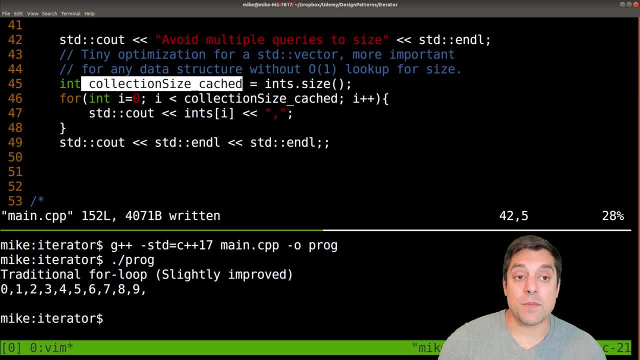 i'm just caching the value of the size so i don't have to recompute it every time, and this is just a very small optimization. but i just want to show you this little trick here because it might be more useful, especially if you've got a data structure that doesn't contain the actual size. 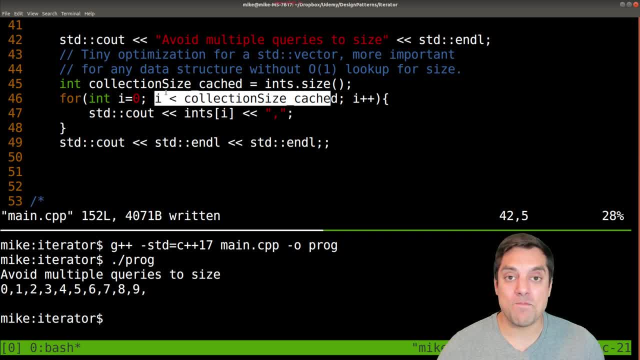 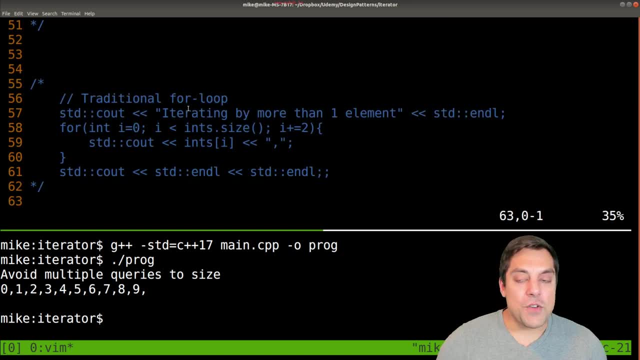 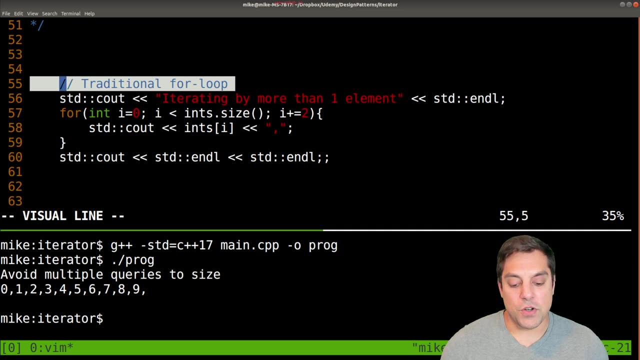 for a, a vector, here. this probably doesn't make that much of a difference, but it's a nice little optimization to know about. so let me go ahead and undo that now. i want to show you at this point something a little bit new with our iteration here, and this is the same traditional for loop that we 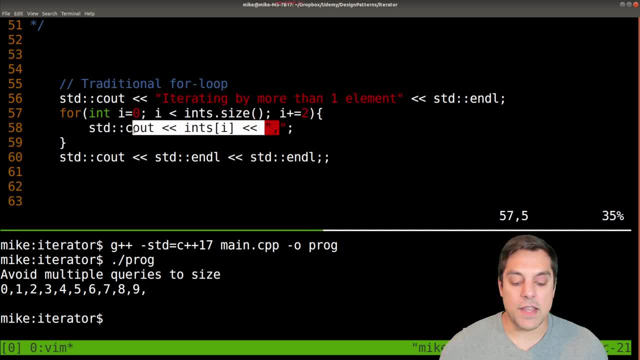 have and we're just taking the size here of our collection and iterating through every element. but what's new here is that we're incrementing by 2 every time. so i'll go ahead and run this example and you'll see that we're just getting half the elements because we're incrementing two items at a time. so at this, 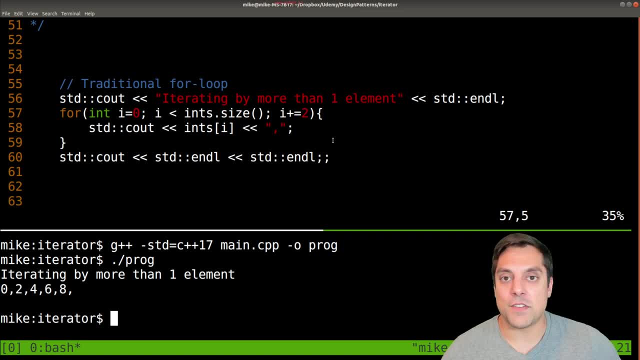 point. you're watching this video and you're saying, well, all this stuff's obvious, we know how to do this in a loop, but what i want to show you, the advantage of iterators is that we don't often know what the intent is of the user from this code. what makes this loop different than what we saw? 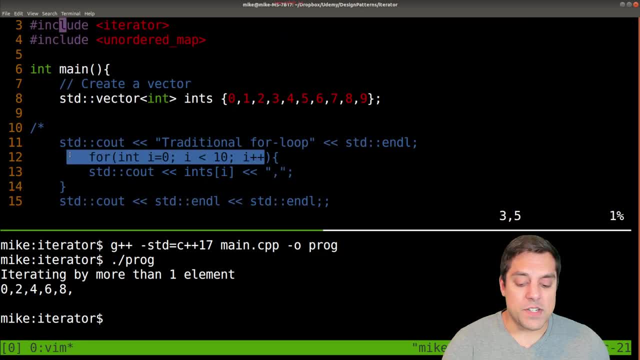 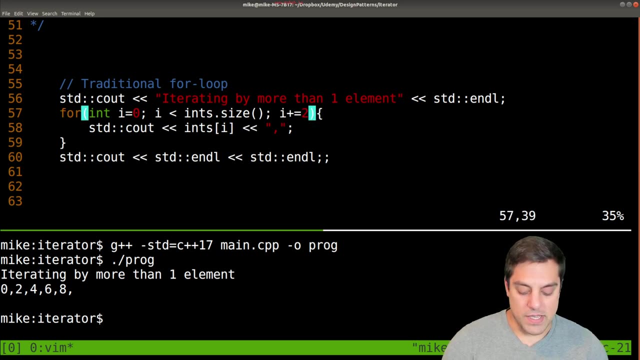 previously. if we scroll all the way up here, where we were just iterating through all the items here in this example in the code, i guess it's clear that we're iterating one item at a time, just as we are also iterating two items at a time. but what stops a programmer from putting in three? or why? well? 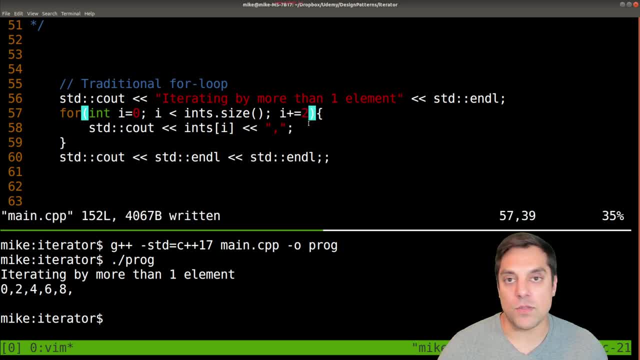 they probably need some sort of comment there to describe why they're hopping two items at a time. if that's your intent, then it needs to be described, or maybe there's a way we can use the structure of our code to make things just a little bit more clear. so let me go ahead and move. 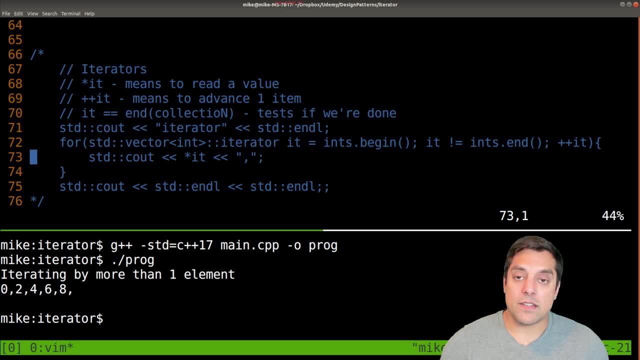 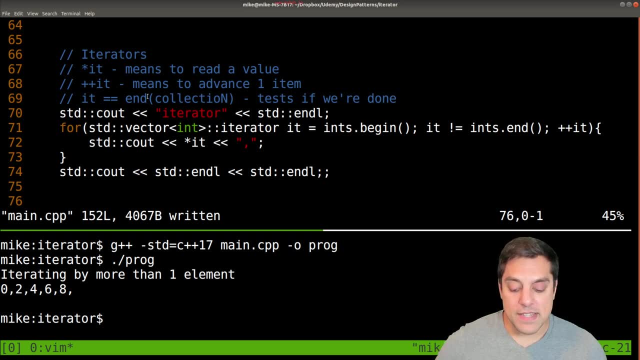 us on here, and now i want to show you the built-in iterators in c++ for the standard library containers. so what do i have here? in this example, i have now an iterator and it's gonna look a little bit funky. but for the actual vector i can get this iterator here. let me go ahead and show. 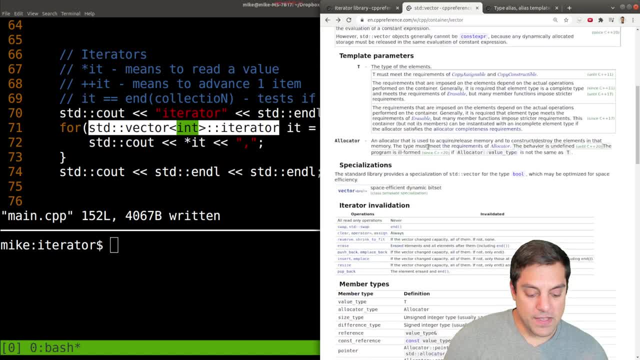 you what that looks like in vector and i'll go down to the iterator here and we can see the different types of iterators, that is, the different types of custom iterators. there are superintendent andısı. that's space, and i have an iterating like sequence看到 on this screen: exactly same thing. 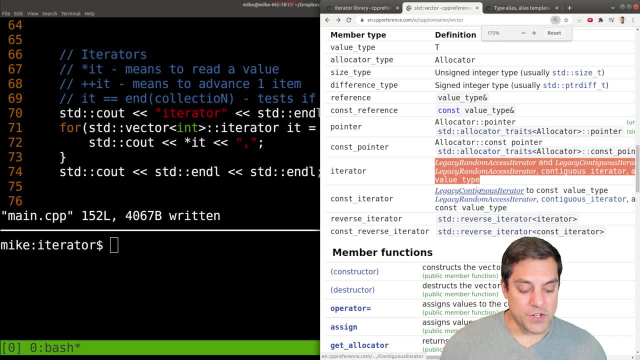 different ways that we can iterate through a particular structure here, whether it's in a contiguous manner, whether it's bi directional, or forward or backward or whatever. These are the different ways that we can have an iterator, And you're also going to see something. 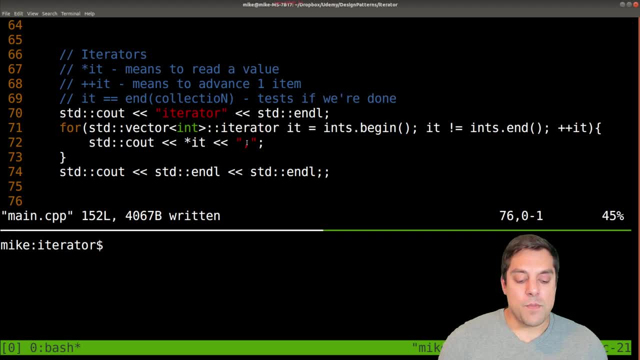 that's a constant writer, which I'll talk about in a moment. But what's neat about this is when I read this line of code- and it is long, but I can fix that in a moment- It describes the intent very clear in the code. what we're trying to do. we're going to start in iterator. 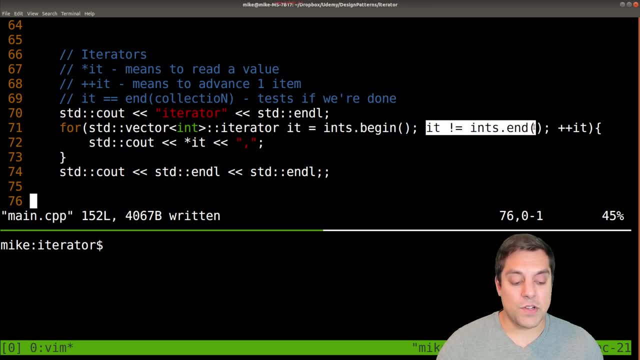 it from the beginning of our collection, And then we're going to look until the end of the collection And then we're going to iterate one item at a time. So it's very clear in the code here that we're intending to look through everything, And you might argue that's. 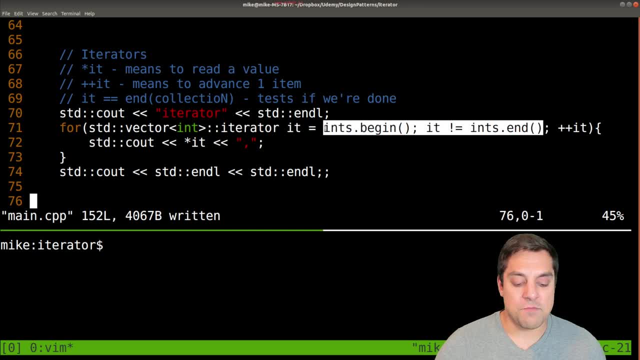 the same thing when you put dot size, but here it's just expressed a little bit more clearly. And then what I'm going to do is print out each value. And since the iterator is a constant, we're going to print out each value. And since the iterator is a constant, 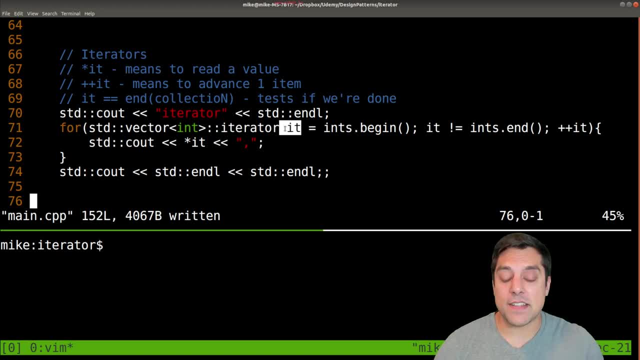 essentially a pointer to the next piece of data in our structure. we dereference it so we can print it out. So in a sense you can think of when I dereference the iterator, that means I'm reading from a value, or perhaps writing as well, And each time through the loop I'm incrementing. 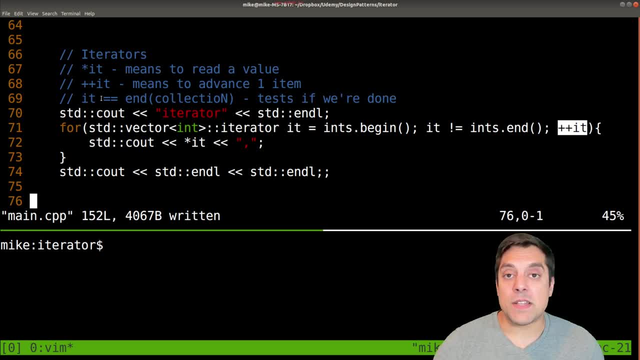 the iterator that's just one at a time, So that means to again move through the collection one item at a time, And I check for the end of our collection, as shown here. And there's a couple ways you can actually do this To use your iterators. you can use something like: 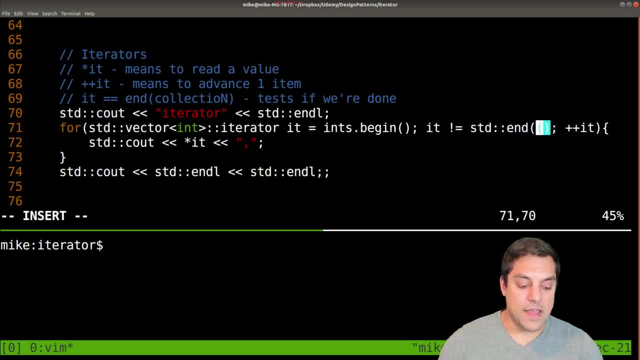 standard end and then provide the collection here, And, but I'm just going to leave it as such here. Okay, so let's go ahead and compile, Let's go ahead and run, And just like that you see the iterator. So again it's a little bit more clear or expressed more in the code what our intent. 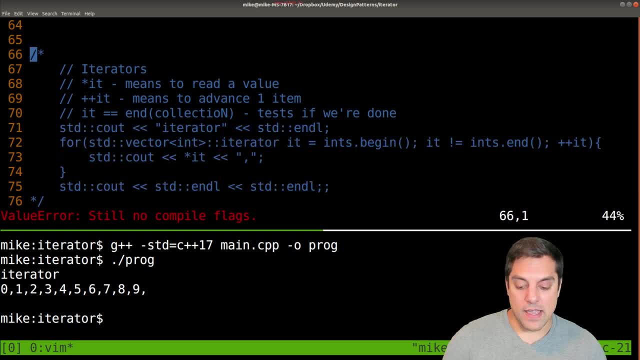 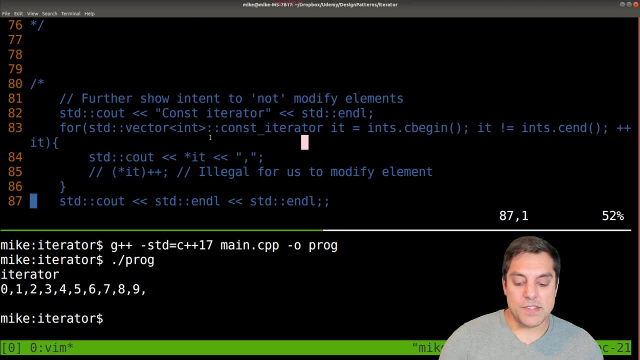 here is with the iterator pattern. Now let me go ahead and move us to our next example. So that's pretty cool, But maybe we're not convinced yet what we can do with iterators. So let's go ahead and show that const iterator. 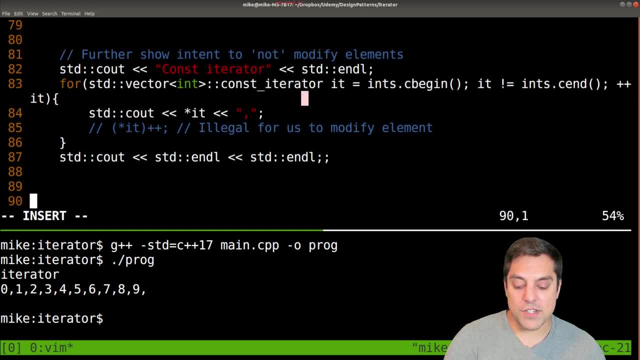 that I told you as a part of vector, And just show you again how this is expressing clearly in the code what we're supposed to do. And this time what's different is I'm supplying const iterator, So that means that I'm not allowed to modify or increment or 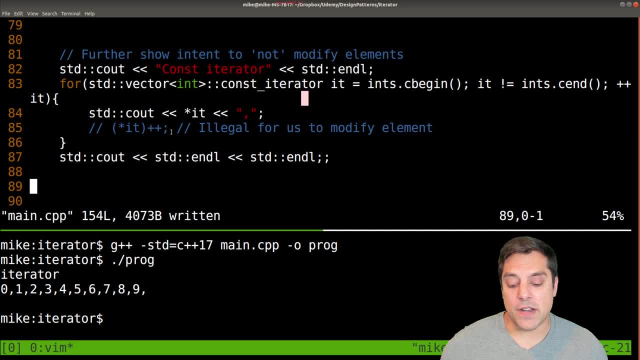 reset, whatever the current element is that I'm pointing to with my iterator here. In fact, if I uncomment this line here, which first I'll run it just to show you that we can in fact iterate through all of our items. But if I try to modify any of these items here, which I'll go ahead and 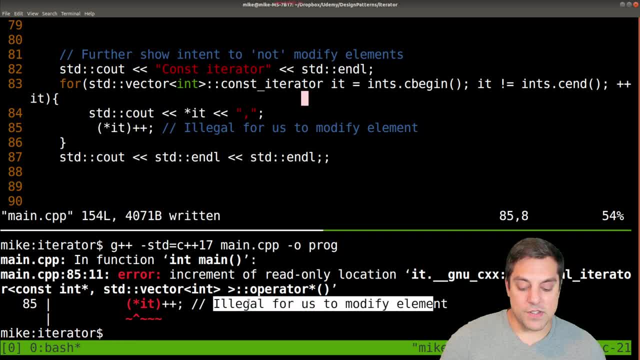 do so, you'll go ahead and see that it's illegal for us to modify this element here. right, It's a read only location, So we can't do that. So, again, we're getting a little bit more powerful in how expressive we are. 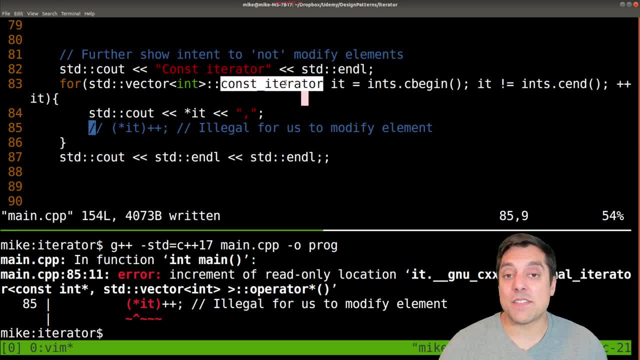 Our code. here with this iterator, we're specifically specifying how we want to iterate through it And we almost have a contract saying that this is const. Now, again, we could do something similar like this in our loop: maybe loop through a collection of data with const or something. But 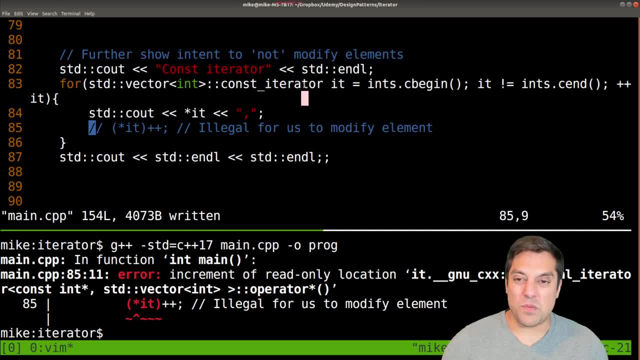 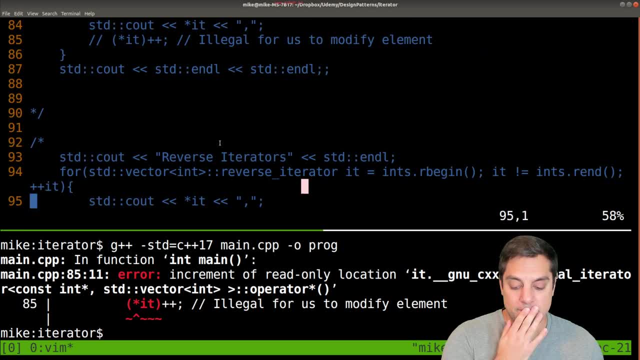 again. this is just very clean to do. So let's go ahead and see if we can add some more power to our iterators, or perhaps see how they can be also expressive in our code. So in this next example I'll show you. 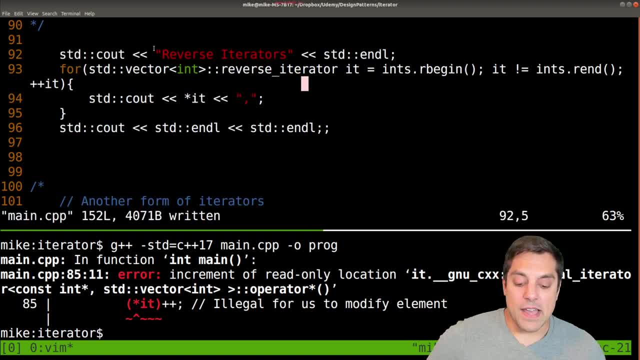 how to do a reverse iterator And in this example, again I'm changing the type of iterator that we have And it's reverse iterator, So you can coordinate. see the pattern here. And this time we're going to start our beginning at our begin, which means, well, the beginnings at the end. 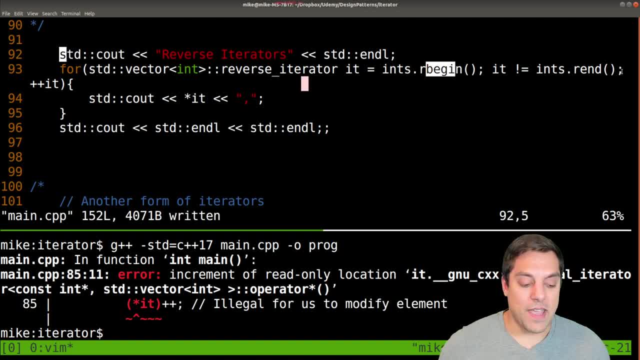 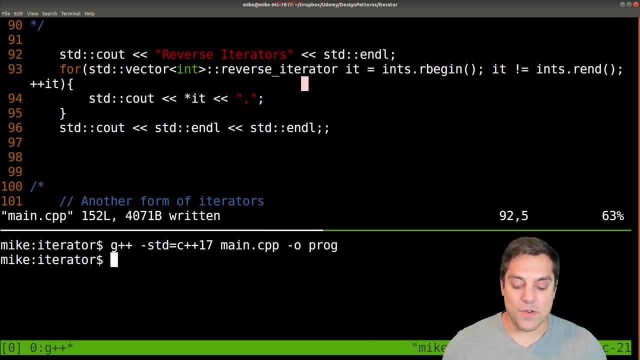 it's reversed essentially. So that's how we set this up And we'll go to the well, whatever the end is, but reverse, So we've just turned things around. So let's go ahead and run the sample, Run our code And you'll see that our elements have indeed been reversed here. So I think that one 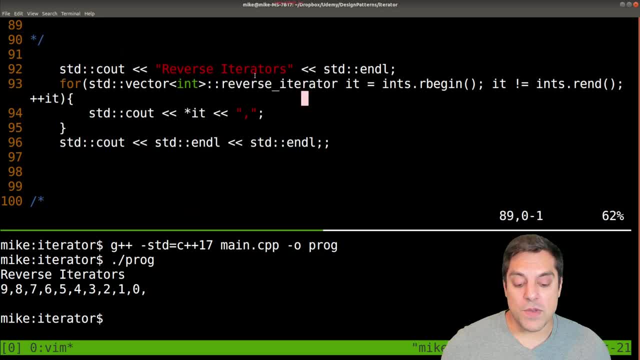 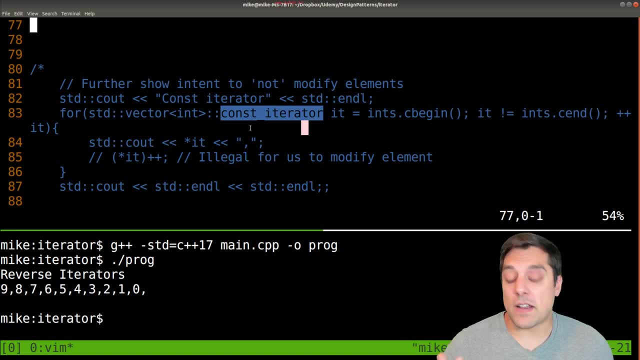 speaks for itself, But again it explains clearly in the code. we can reverse through our iterators, return a iterator that goes forward one element at a time, but we're not allowed to modify them or just iterate like we previously were with the loops. So I think that's pretty cool. 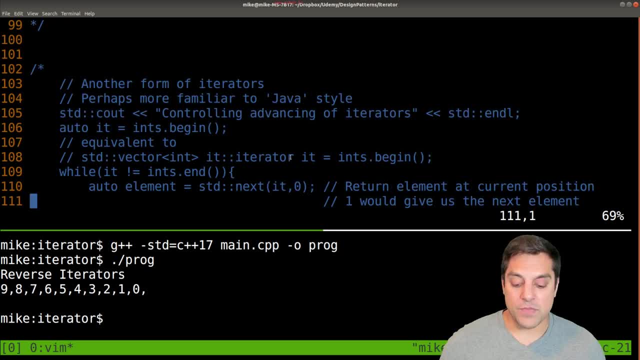 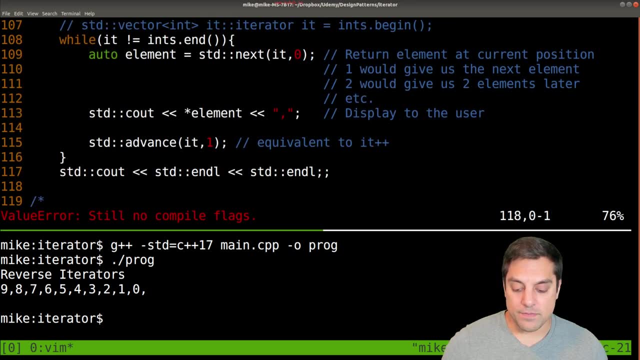 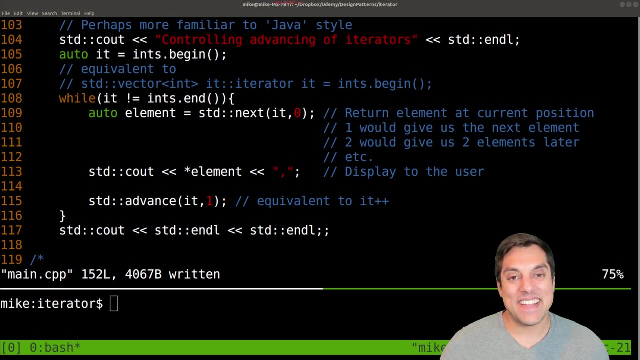 Okay, but we still have some more power here with our iterators in how we advance. So let me go ahead and show you another example here, And I'll make this bigger so it can fit on the screen here. And in this example I say it's almost a Java like example. 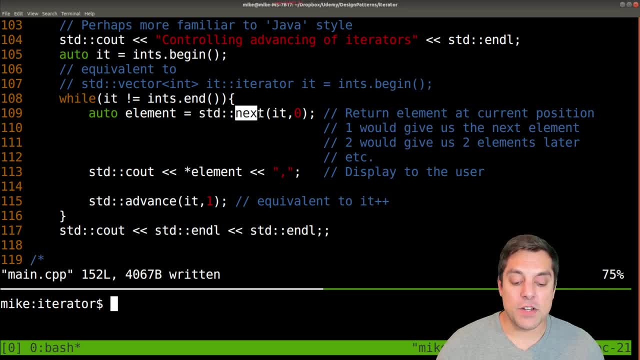 because we actually do in C++ have these functions for the next item or grabbing the next element or advancing. So in Java you might have next or pre, or maybe you've seen some of these functions in that standard library. Haven't, don't worry about it, But we're going to go ahead and do that. 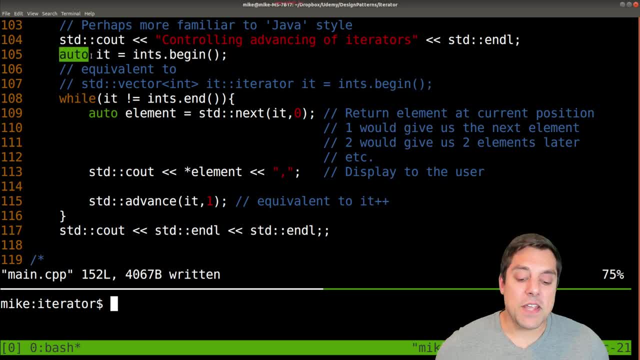 We have those available in C++. So in this particular example, I'm creating an iterator here And I'm just using auto to do the type deduction Because, again, sometimes it's a lot to write out the full iterator for a type, though typically I like to do that because I like to be 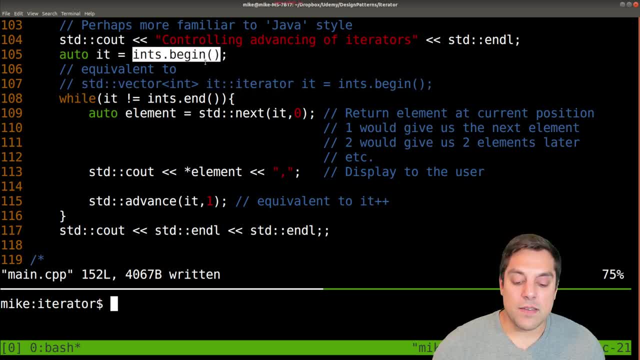 explicit in my code. But then we just have the beginning here, iterator, And I just have a while loop here that says, well, we're not at the end. whatever, the current element is zero. or rather the next function is doing is saying from our iterator, grab us the item that's how many? 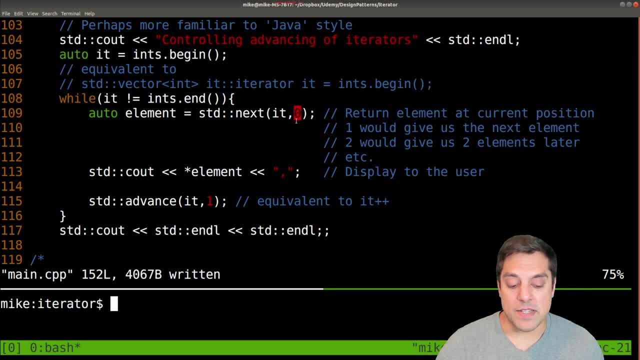 positions offset And if it's zero, that'll be the current element. If it's one, it'll look forward to the next element. then we'll just print it out And then we can advance our iterator. And this is equivalent to doing the I plus plus that we were doing earlier in our loops, except I'm able. 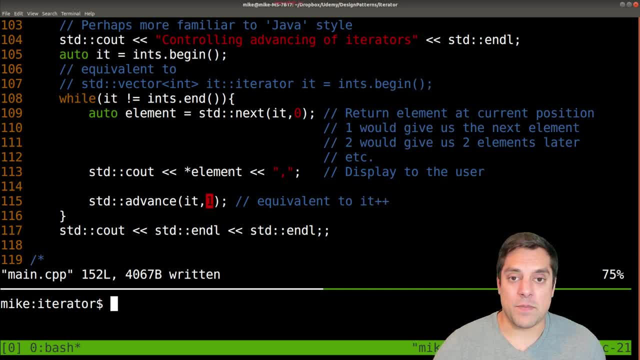 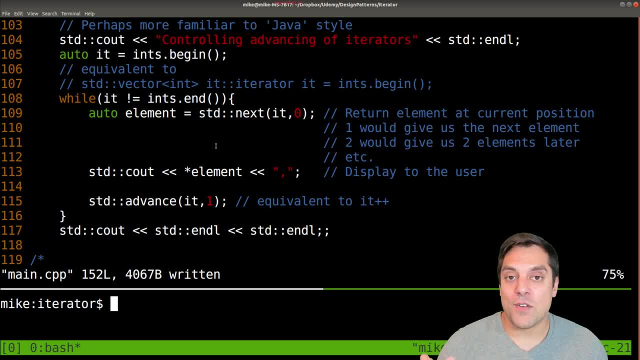 go ahead and do that, And then we're going to go ahead and do that, And then we're going to go, because usually you're looking through a sequential data structure, one element at a time. But what if you have a tree? What if you have a graph or some other structure? So this is where it's really. 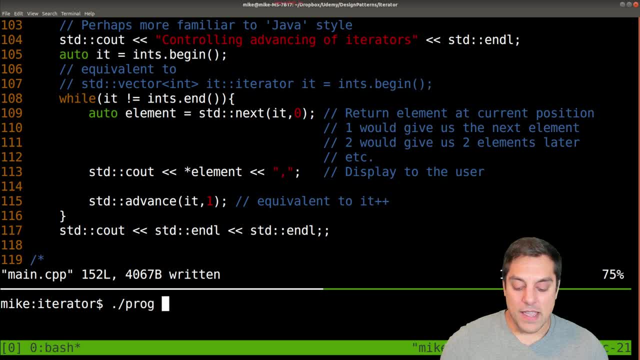 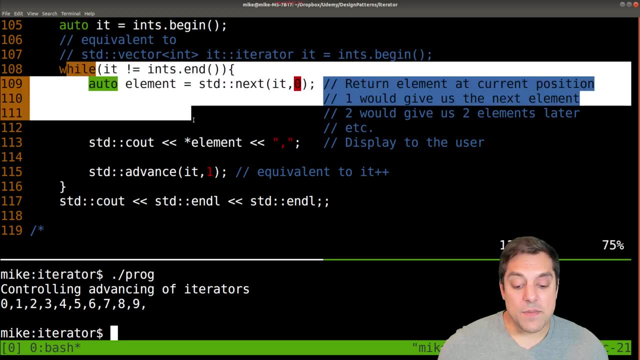 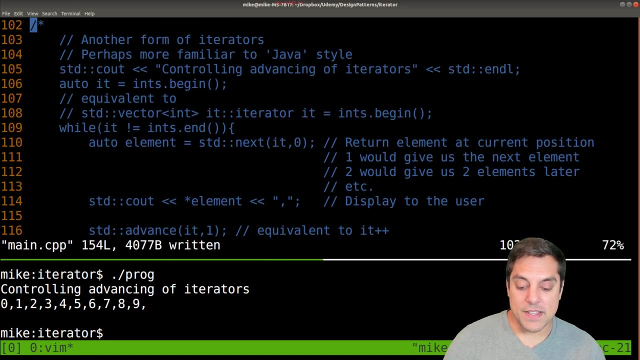 handy. So let me go ahead and just compile this and run it So you can again see that we have our pattern here, just as we previously have done. So this can be another very expressive way to iterate in advance through our code. So I'll go ahead and return this and look at yet another example here. 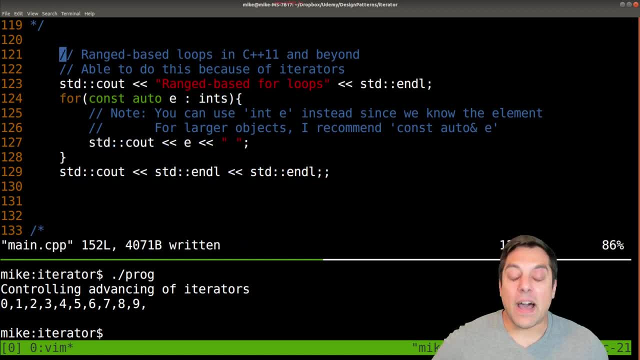 Now what implementing your own iterator buys you, or why it's sort of useful or nice to have, especially if you're using the standard data structures. you get these with the standard template library. the C++ STL is you can write range based for loops like this. So in this 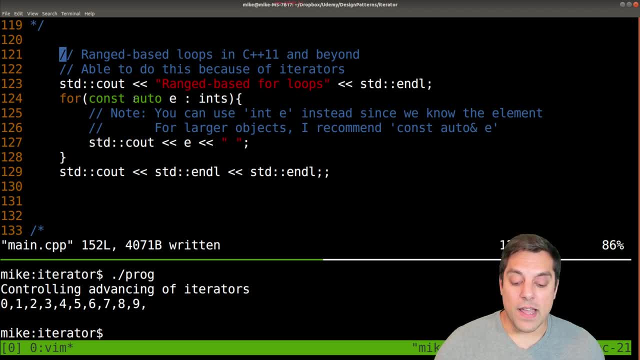 example, I've written a range based for loop where I can just iterate through some collection ints, which was my original vector, and each of the elements I'll refer to as E And I'm going to make them constant. So I'm going to make them constant, And I'm going to make them constant. 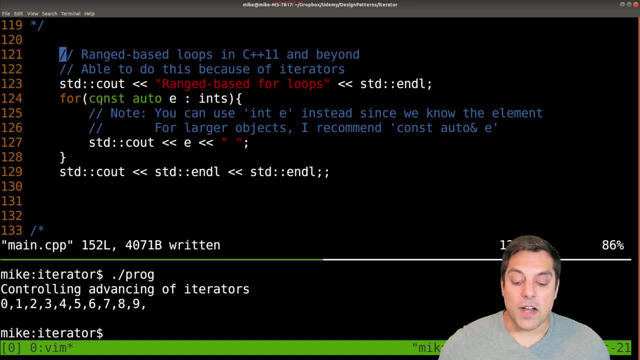 So that they cannot be modified. So this is our const iterator here. So let me go ahead and run this, just so you can see the example. And again using a range based loop. And again, when I write this type of loop, it's very clear that I'm not trying to skip through every other element or anything. 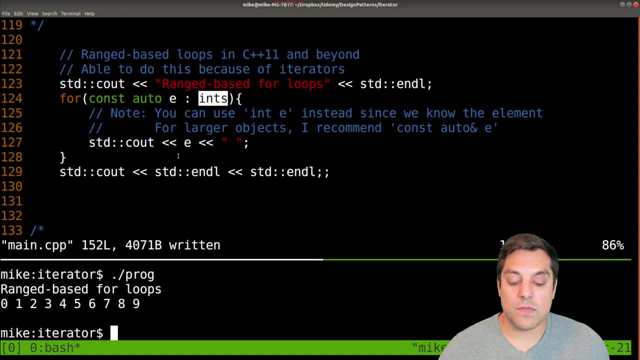 I'm saying, for every element in this collection, execute this code here, which is essentially just print everything out. So again, I like that expressiveness, this description, and I'm going to make sure that it describes my intent very clearly, that I'm looking through the entire range here of 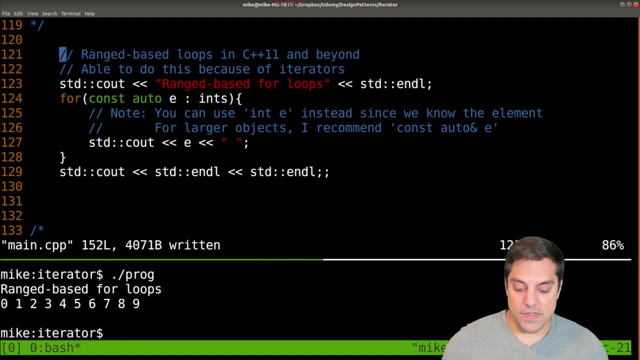 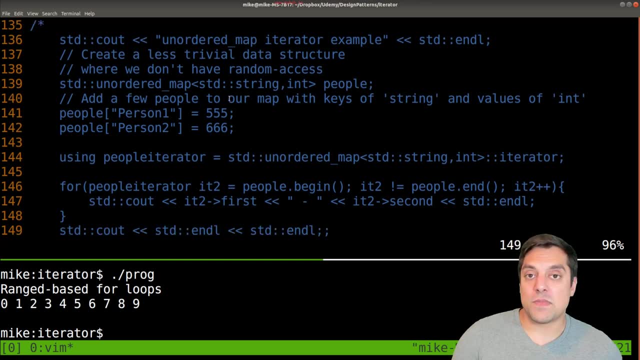 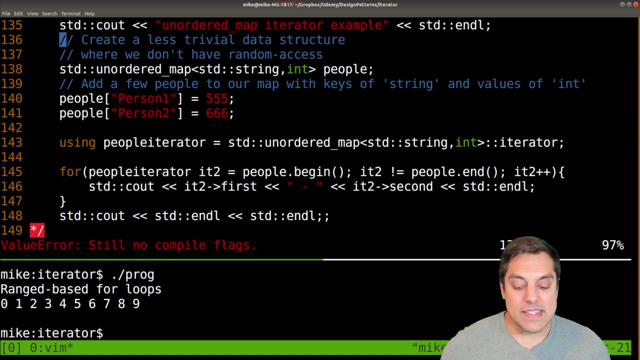 my collection. Okay, so, with that said, let's go ahead and look at another example here, And this time I'm going to go away from the vector, which we've previously been doing, and look at an unordered data structure. This will be the last example here in the video, But the idea is: 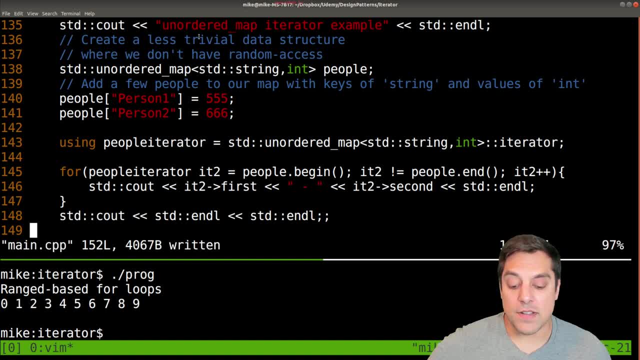 this time I have a map data structure and specifically an unordered map. So, again, the order isn't necessarily clear, But we might want to traverse and see all the keys in our specific data structure, for instance. And how can we do that? Well, we need to use some iterator. 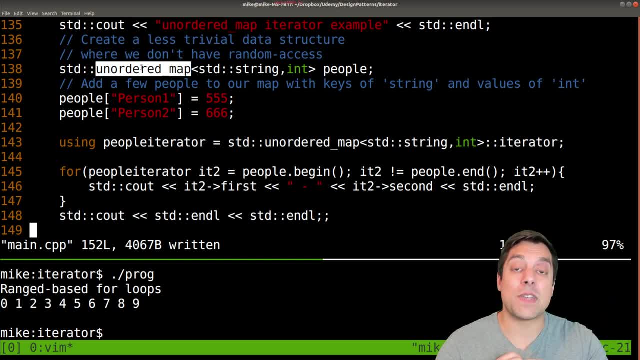 something that's going to tell us how do we traverse through this data structure so we can eventually see everything. As often we might want to iterate through a map and put it in some other data structure and manipulate it in some other form, So this is our option here. So what I'm 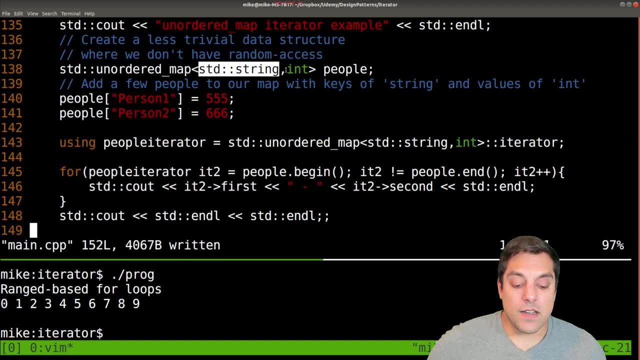 going to do is create an unordered map here with a key of a string and a value of an integer, And I'm just going to call these people. So we have somebody's name and maybe their phone numbers here. Okay, so person one and person two. Now a little trick here if you do get tired of writing. 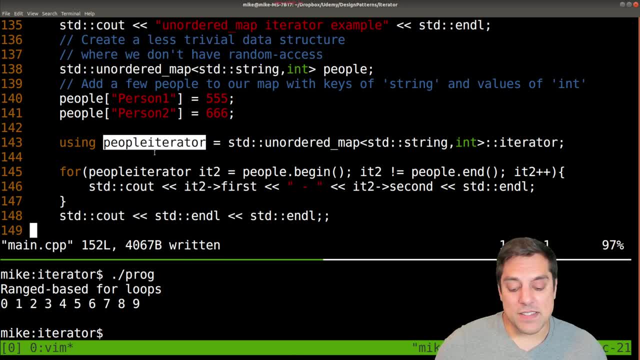 out these iterators here is: you can use a type alias here, So I'm just going to refer to people iterator as this whole thing here, So the type of the or the template arguments of the type of the unordered map, so the key and the value pair and an iterator, I'm just going to call it people. 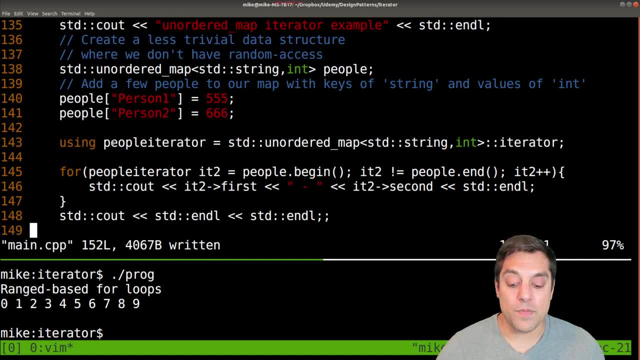 iterator. So you should just be aware that you might see this in larger code bases. If you see types that you're not aware of that and they have some sort of iterator title in them, they're probably using this trick here And again. if you're not familiar with it, you can look at type. 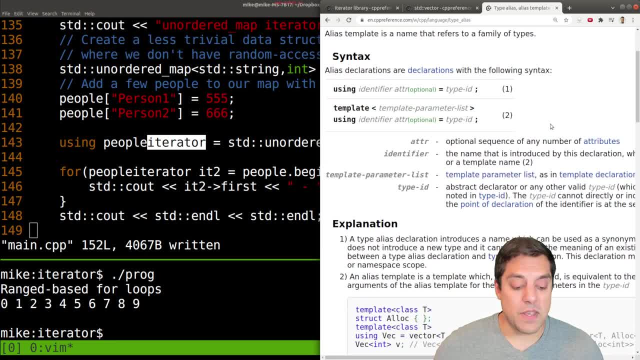 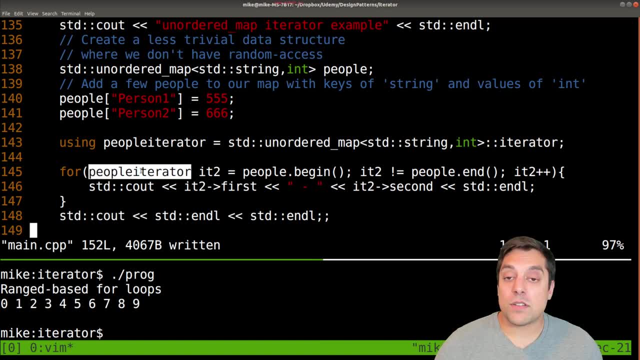 aliases which have been available in C++ 11 and beyond, just to see how they're used with the using keyword here. Okay, so how do we do that? Well, we're going to go ahead and create an iterator. So how do we use this? Well, just like we previously did, and this time just using a. 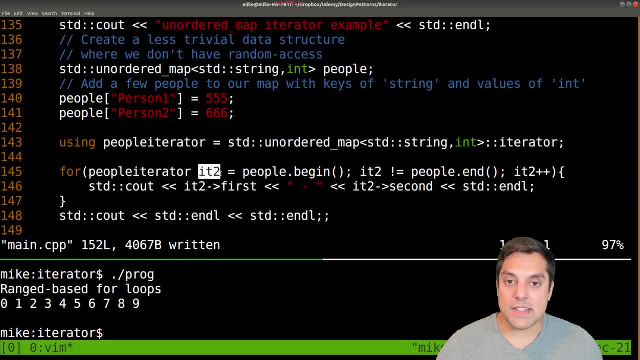 for loop. we have our people iterator- and I've just called this it to we start at the beginning, and we're going to go till the end here, of our people collection here, which is, these two key value pairs and increment one at a time. Okay, so let's go ahead and see what this gives us. So if 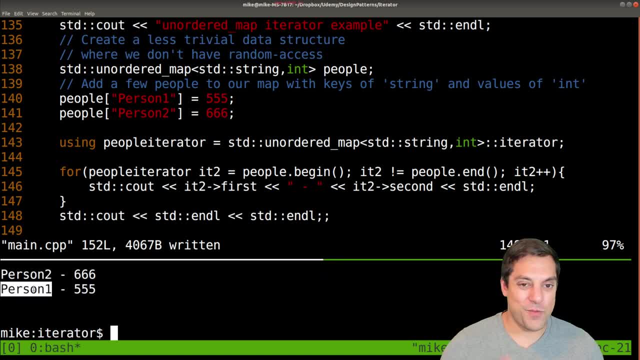 I run this, I'll get person two and then person one, which is a little bit interesting that we have that traversal, considering we added them in this order. But again, that tells us something about how we sequentially access something in this unordered map data structure, which is some sort of hash map. 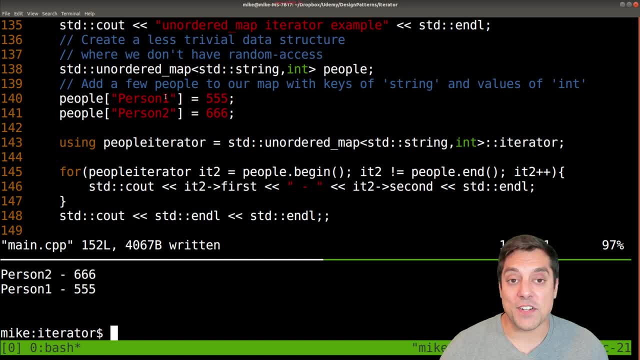 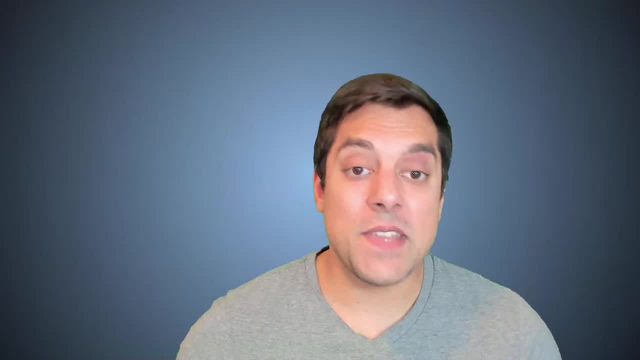 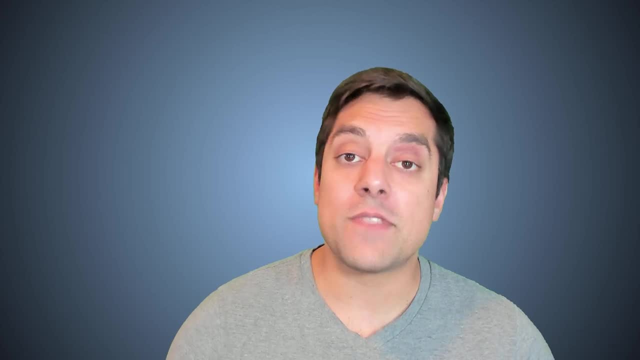 algorithm And if you have a tree or some other data structure, you'll also get perhaps a different traversal. So, with that said, that's iterators. So in this video we've looked at a behavioral design pattern, the iterator, And it's again a way to traverse through some sort of data. 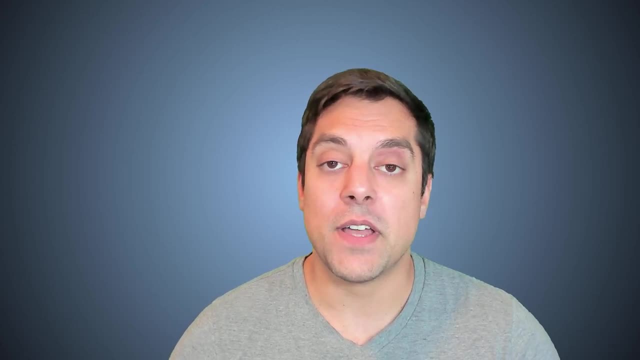 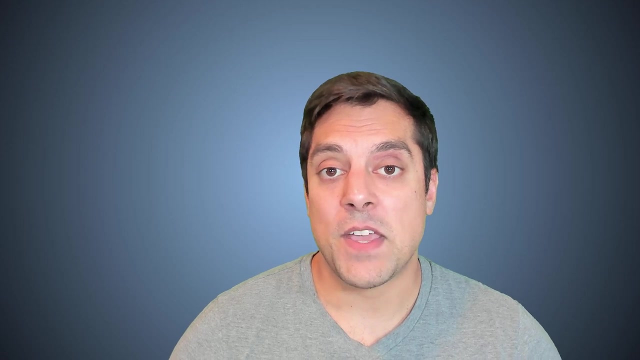 data structure, whether it's array based or some linked data structure, in a consistent or uniform manner And you can have different iterators to traverse a data structure in different manners. we'll look at in the future perhaps folks like in the comments to see how to build iterators of. 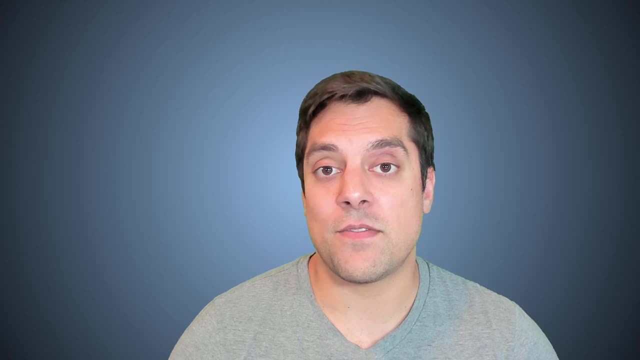 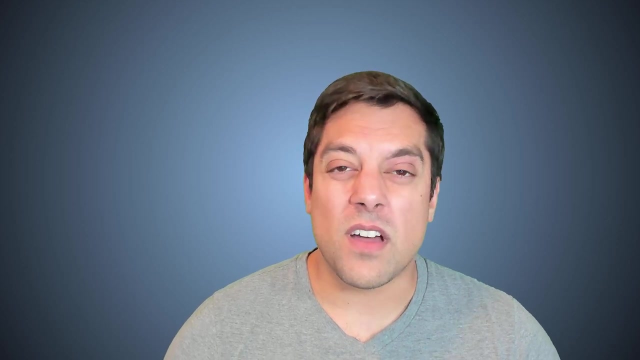 your own So you can see how to take advantage of some of the language constructs like range based loops. But I hope we'll encourage you stylistically to write iterators when you want to write good code. that is very expressive about what the intent is. 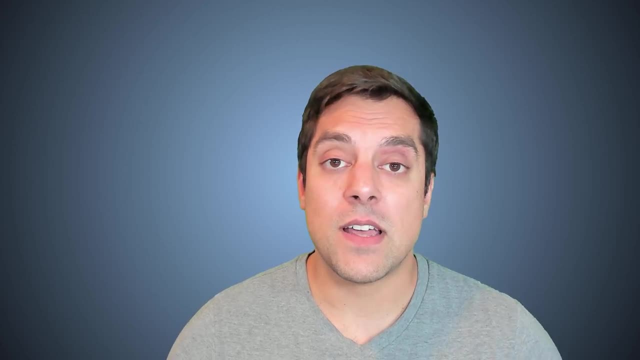 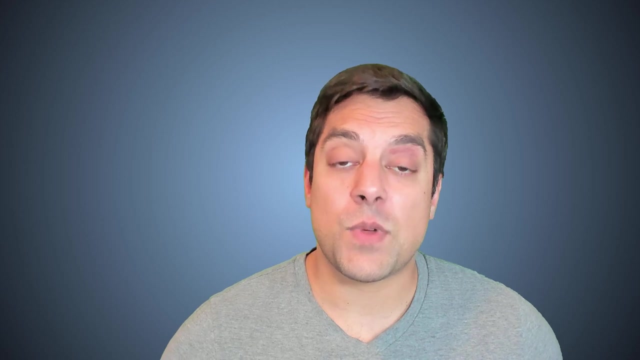 of what you're doing. You think iterators might be a little bit too heavyweight. Well, you can always profile and try to optimize later and try to use raw loops if you truly need. But at the least, what I'll also say is that iterators are important to know about because a lot of the standard